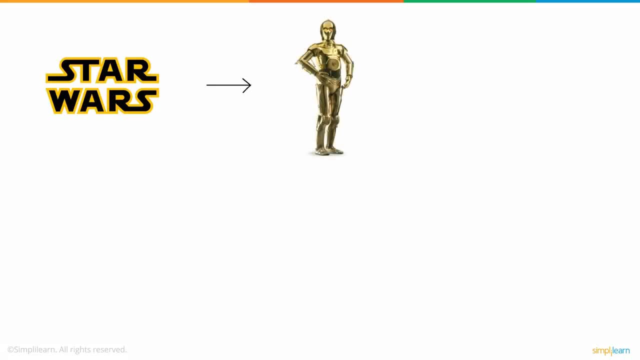 Star Wars fans would be familiar with the golden, life-sized hospitality robot C-3PO. While Star Wars might be set in a galaxy far, far away, the reality of having machines talk and respond to us in a human-like manner is already a reality which keeps getting more. 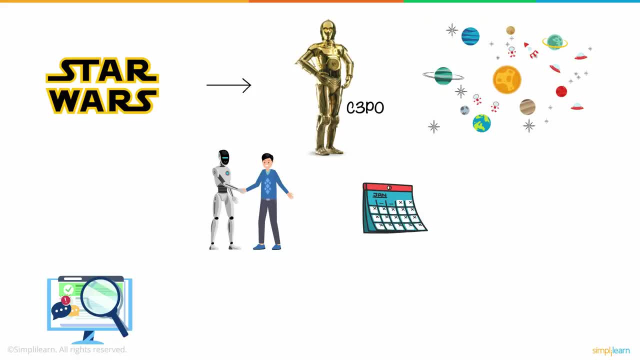 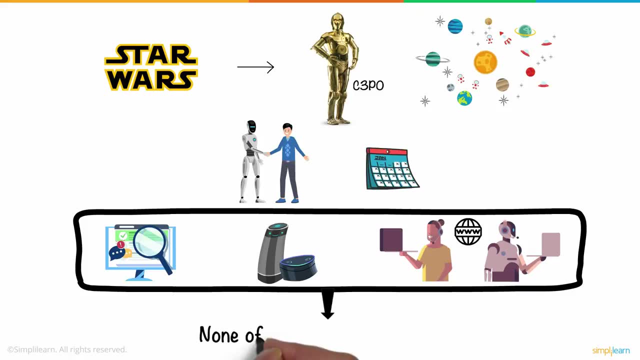 and more realistic with every passing day. The people you ask for queries on websites, your smart assistants, even calls made over the internet, all of them have one thing in common: None of them are actually human. Now, you must be thinking if they are not human, 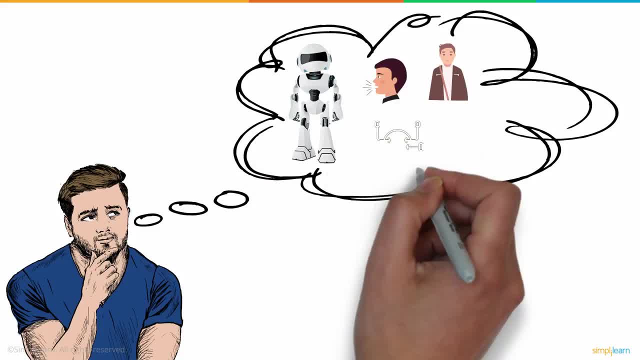 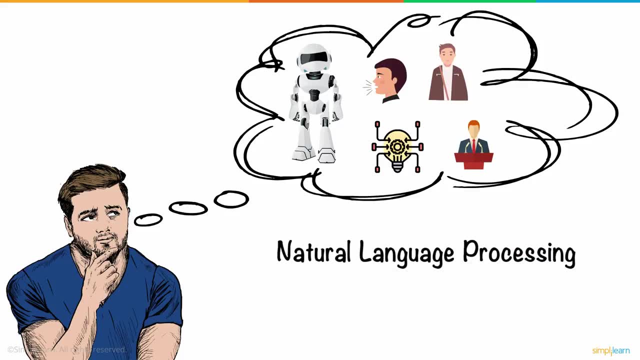 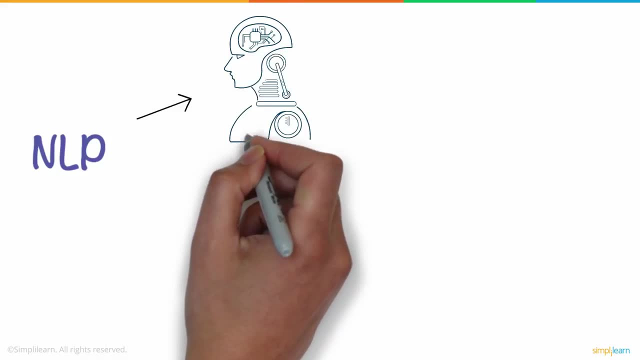 how do they manage to sound and seem so human-like, How do they respond to me so intelligently And how are they so articulate? This, my friends, is the magic of natural language processing. What is NLP? Natural language processing or NLP, refers to the branch of artificial 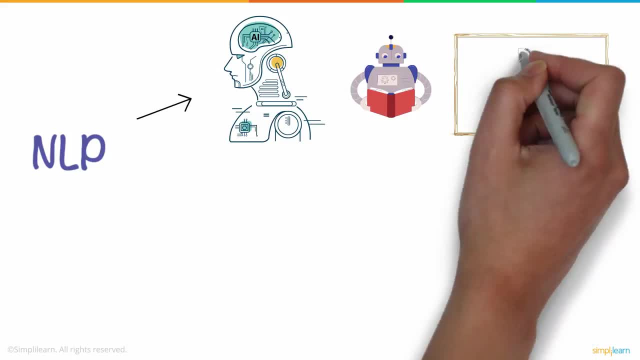 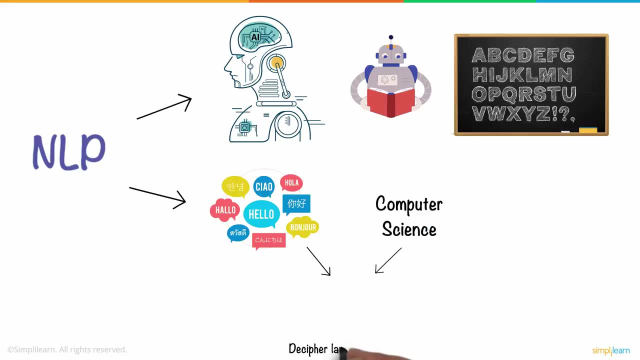 intelligence that gives the machines the ability to read, understand and derive meaning from human languages. NLP combines the field of linguistics and computer science to decipher language structure and guidelines and to make models which can comprehend, break down and separate significant. 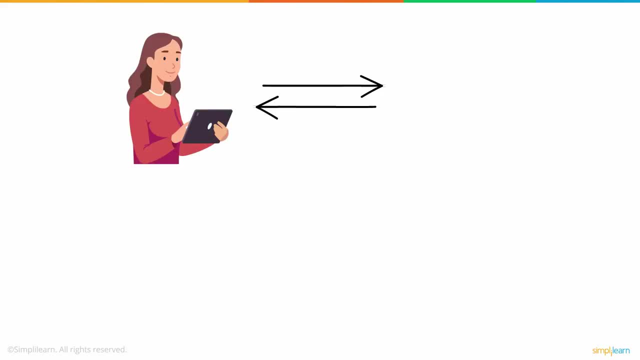 details from text and speech. Every day, humans interact with each other through public social media, transferring vast quantities of freely available data to each other. This data is extremely useful in understanding human behavior and customer habits. Data analysts and machine learning experts utilize this data to give machines the ability to read, understand. 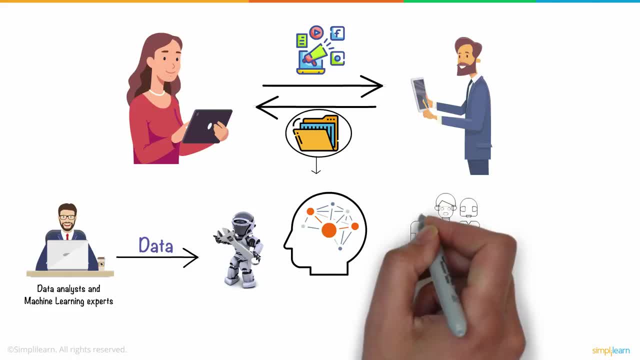 and understand. This data can be used in a variety of ways. and it can be used in a variety of ways. NLP has the ability to mimic human linguistic behavior. This helps save millions in terms of manpower and time, as you don't need to always have a person present at the other. 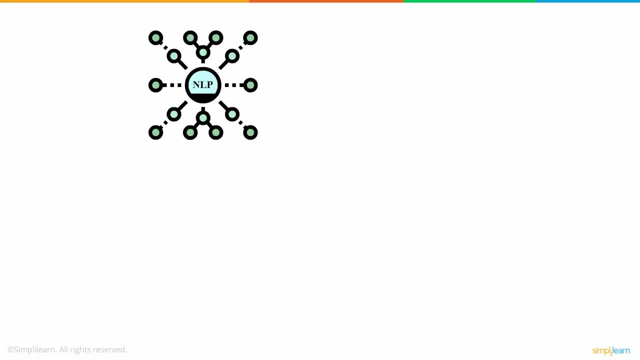 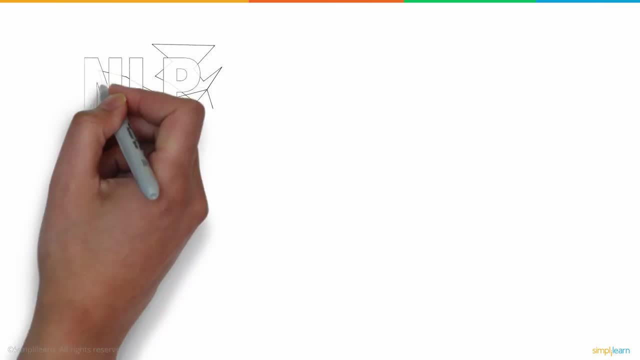 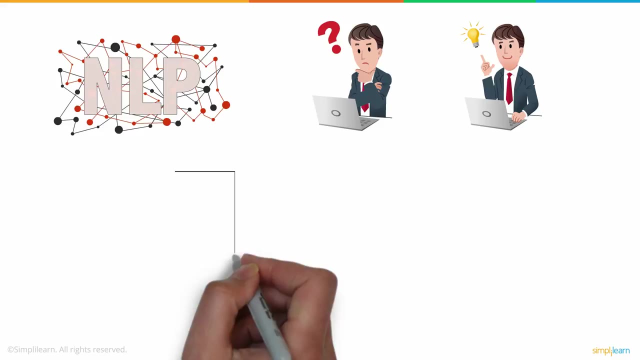 The NLP genesis app will search through the web and find any cases of published documents which may match your work line by line. While NLP seems really cool, yet a cutting-edge and complicated technology concept, it is actually pretty easy to learn. You start off. 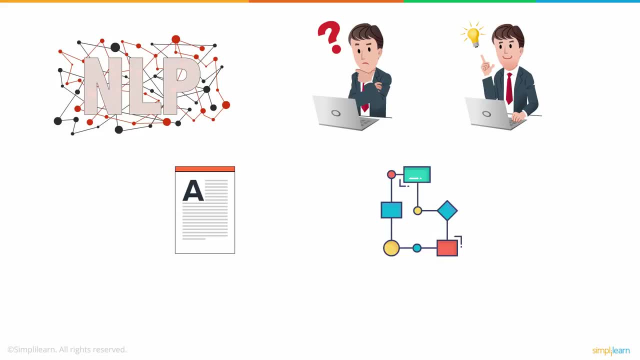 with a document or an article. To make your algorithm understand what is going on in it, you need to process it into a form which is easily comprehensible by the machine. This is no different than making a child learn to read for the first time. 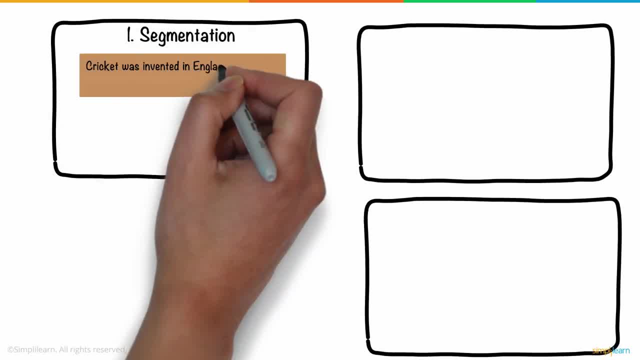 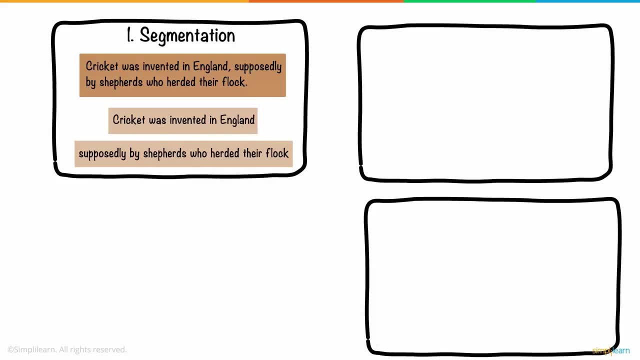 You start off by performing 19 concerning devices. That's a little complicated when segmentation, which is to break the entire document down into its constituent sentences, You can do this by segmenting the article along its punctuations like full stops and commas, For the algorithm to understand these. 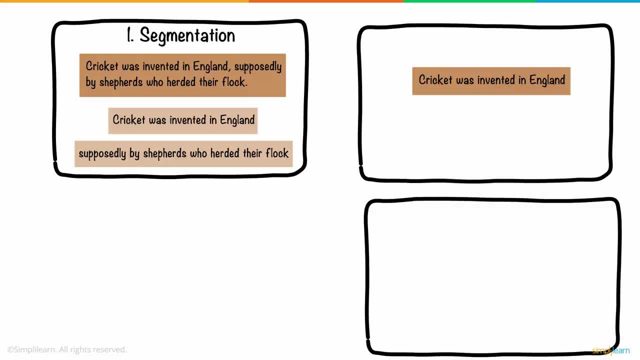 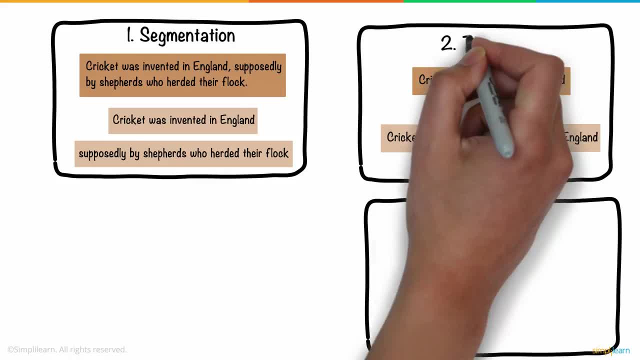 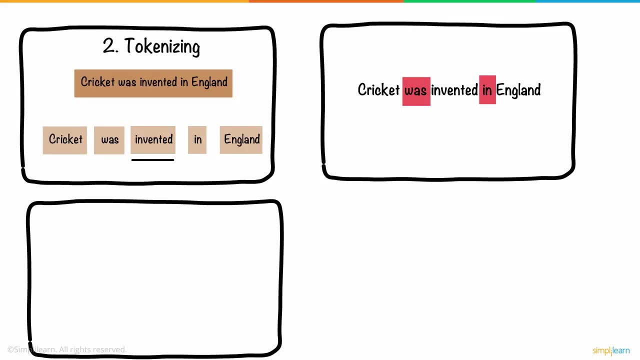 sentences. we get the words in a sentence and to explain them individually to our algorithm, So we break down our sentence into its constituent words and store them. This is called tokenizing, where each word is called a token. We can make the learning process faster by getting rid of non-essential words which do not 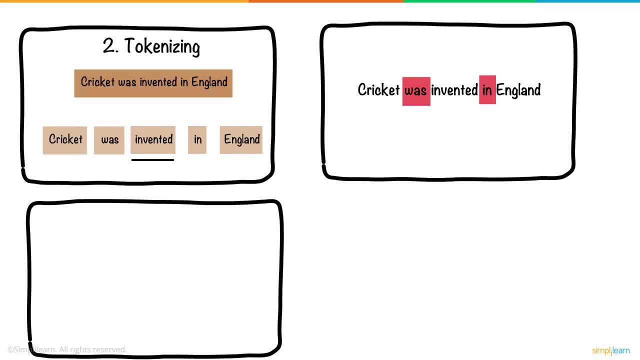 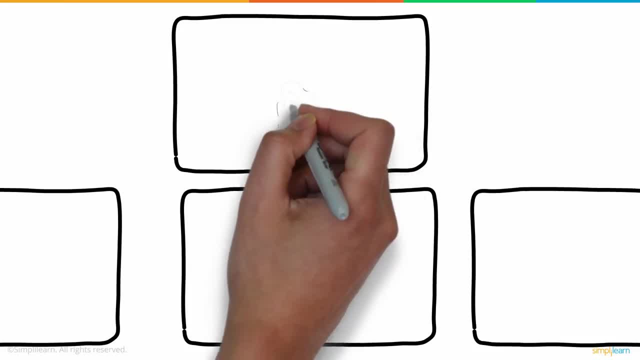 add much meaning to our statement and are just there to make our statement sound more cohesive. These words, such as are and the, are called stop words. Now that we have the basic form of our document, we need to explain it to our machine. We first start off by explaining that some words like skipping, skips 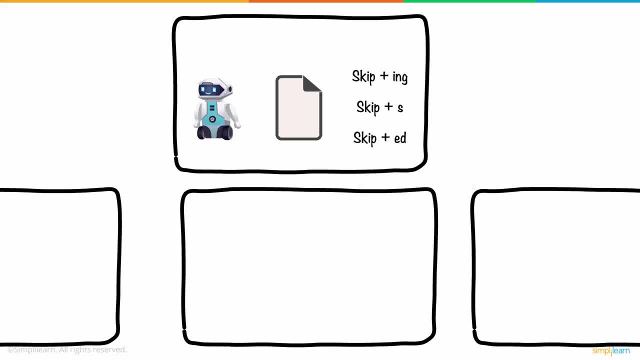 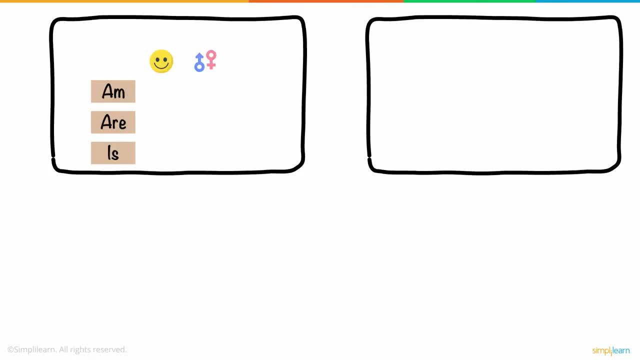 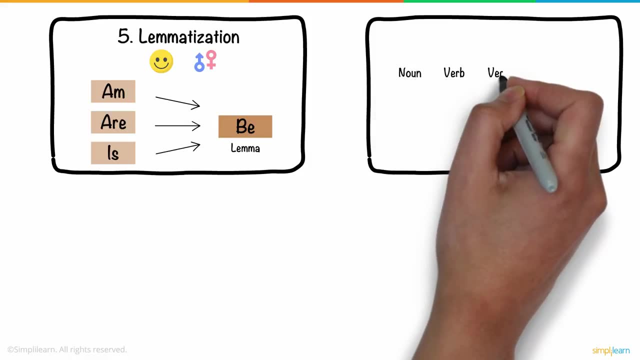 skipped are the same word with added prefixes and suffixes. This is called stemming. We also identify the base words for different word, tense, mood, gender, etc. This is called lemmatization, stemming from the base word lemma. Now we explain the concept of nouns, verbs. 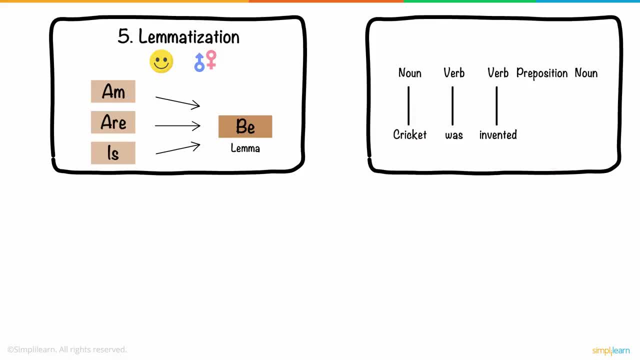 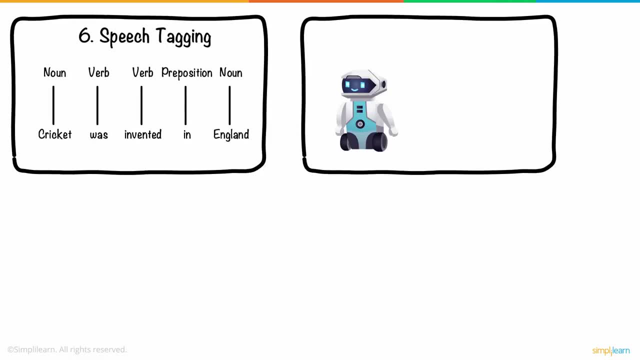 articles and other parts of speech to the machine by adding these tags to our words. This is called part of speech tagging. Next, we introduce our machine to pop culture references and everyday names by flagging names of movies, important personalities or locations etc. that may occur in the document. This is: 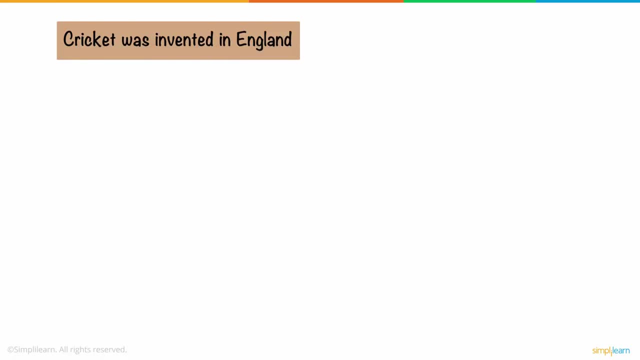 called named entities. Once we have our base words and tags, we use a machine learning algorithm like Naive Bayes to teach our model humans, sentiment and speech. At the end of the day, most of the techniques used in NLP are simple grammar techniques. 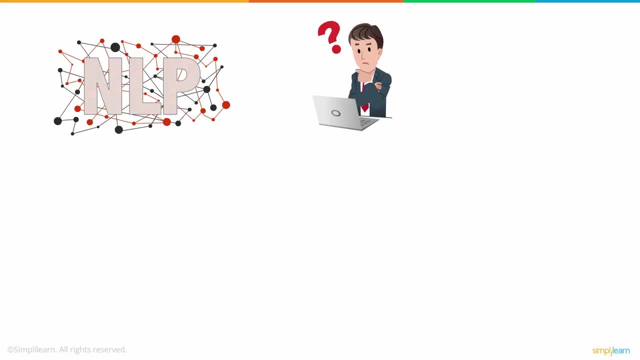 While NLP seems really cool, yet a cutting edge and complicated technology concept, it is actually pretty easy to learn. You start off with a document or an article. To make your algorithm understand what is going on in it, you need to process it into a form. 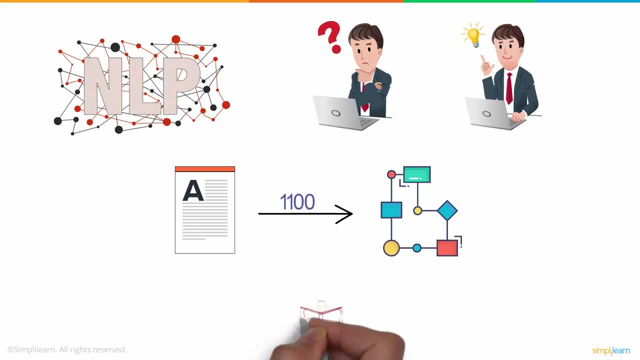 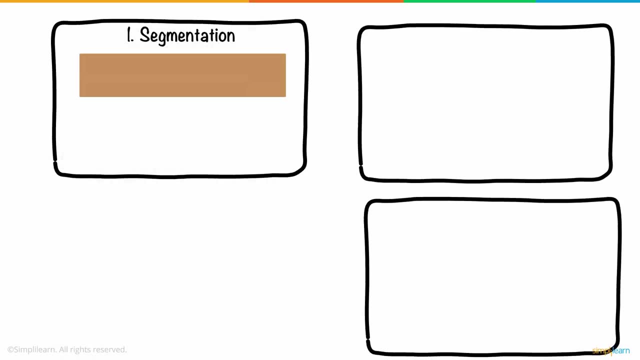 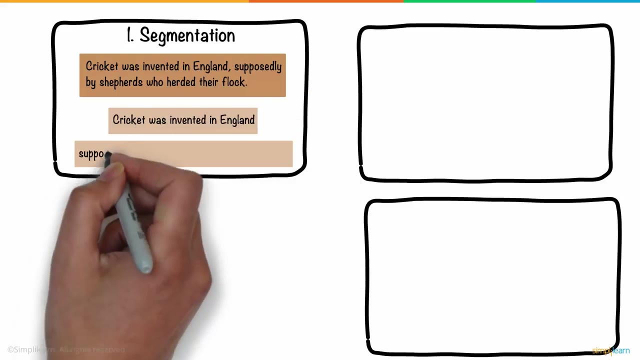 which is easily comprehensible by the machine. This is no different than making a child learn to read for the first time. NLP can also be used to perform segmentation, which is to break the entire document down into its constituent sentences. You can do this by segmenting the article along its punctuations. 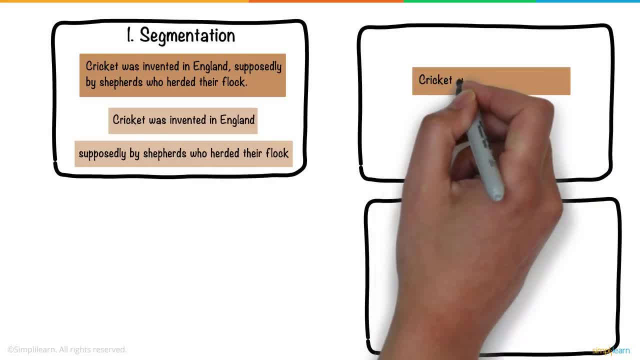 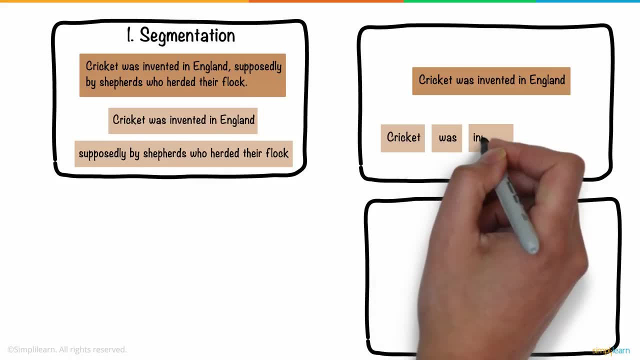 like full stops and commas, For the algorithm to understand these sentences. we get the words in a sentence and to explain them individually to our algorithm, So we break down our sentence into its constituent words and store them. This is called tokenizing, where each word 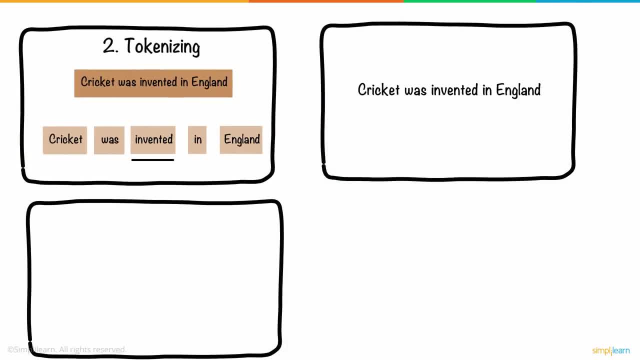 is called a token. We can make the learning process faster by getting rid of non-essential words which do not add much meaning to our statement and are just there to make our statement sound more cohesive. These words, such as are and the, are called stop words. 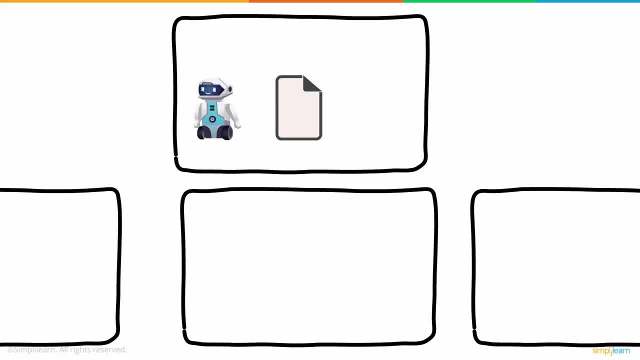 Now that we have the basic form of our document, we need to explain it to our machine. We first start off by explaining that some words like skipping, skips, skipped, are the same word with added prefixes and suffixes. This is called stemming. We also identify the base. 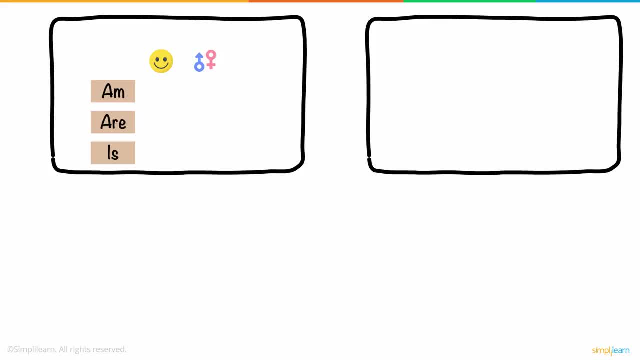 words for different word-tents: mood, gender and gender. If we use the letter t as the starting letter in the sentence, the added prefixes will be the same as the starting letter on the letter-tent Now raising. our machine will interpret all words by adding tags to our document. This: 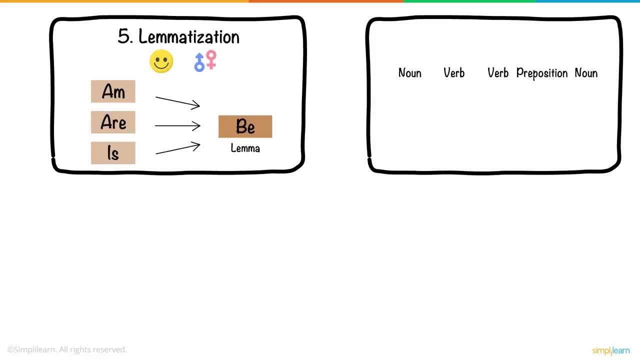 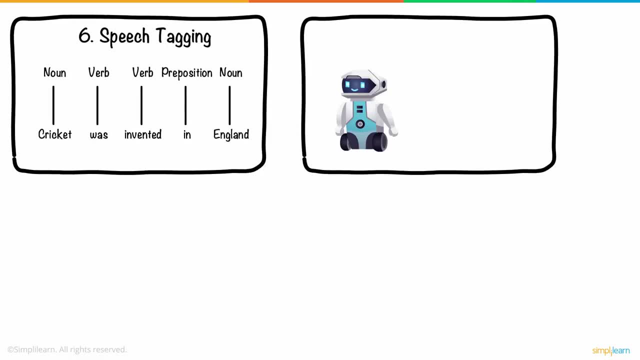 is called lemmatization, stemming from the base word lemma. Now we explain the concept of nouns, verbs, articles and other parts of speech to the machine by adding these tags to our words. This is called part of speech tagging. Next, we introduce our machine to pop culture references and everyday names by flagging. 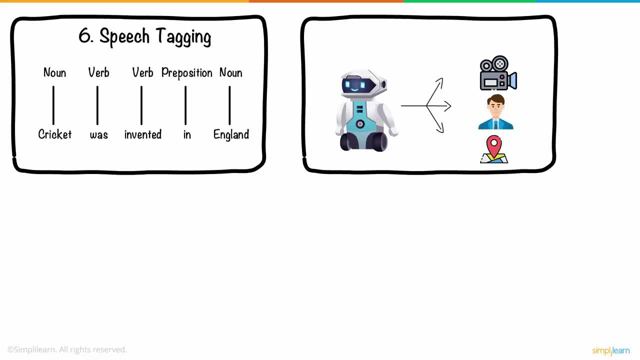 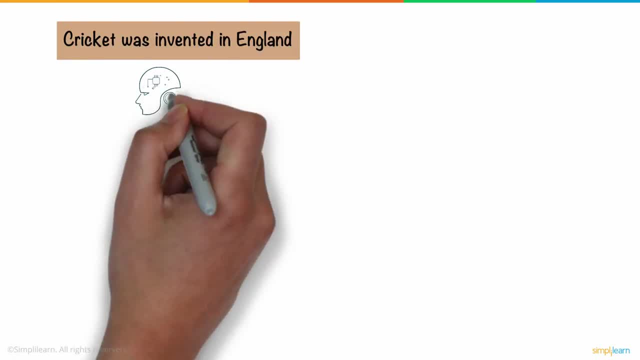 names of movies, important personalities or locations etc. that may occur in the document. This is called named entity tagging. Once we have our base words and tags, we can add and tags. we use a machine learning algorithm like Naive Bayes to teach our model humans.